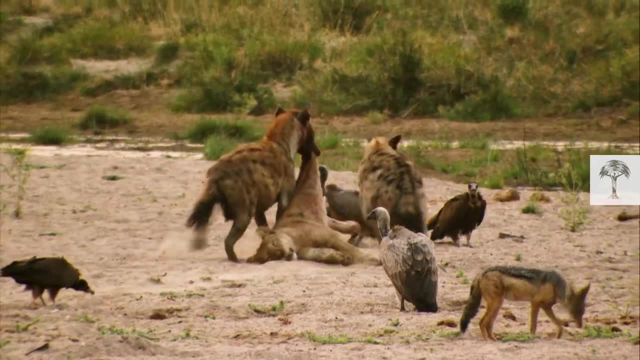 contained within carcasses, which helps prevent the spread of diseases. This doesn't just make the environment look nicer: As they eat, scavengers get rid of bacteria contained within carcasses, which helps prevent the spread of diseases. This doesn't just make the environment look nicer: As they eat, scavengers get rid of bacteria contained within carcasses, which helps prevent the spread of diseases. 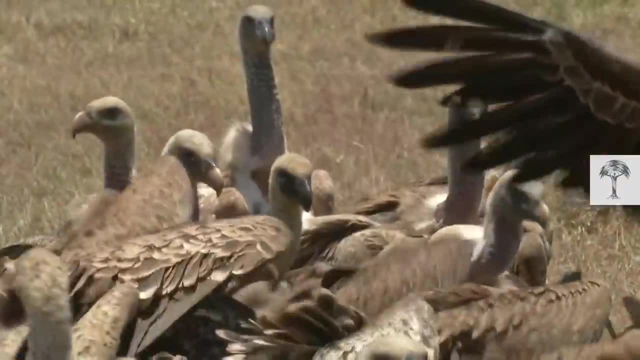 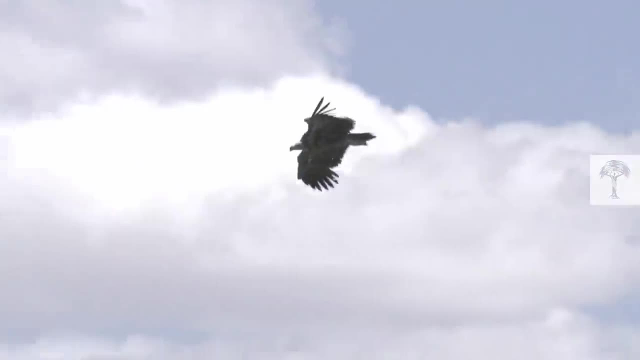 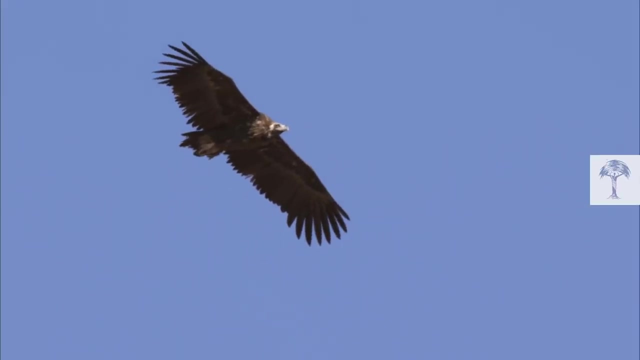 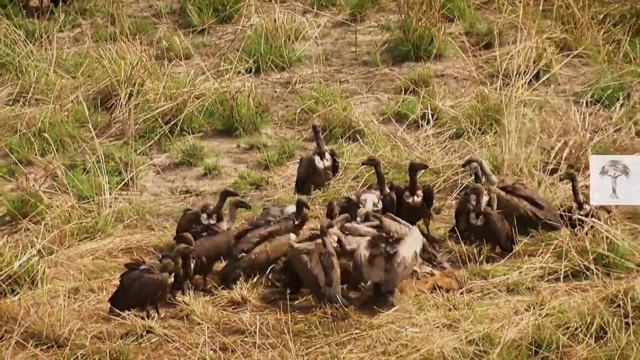 Vultures are especially good at this. Their strong stomach acid kills off toxic bacteria like anthrax and botulism And thanks to their ability to fly high and spot dead animals over long distances, they're usually the dominant scavengers in an ecosystem. In Africa, vultures clear up to 70% of all carrion. 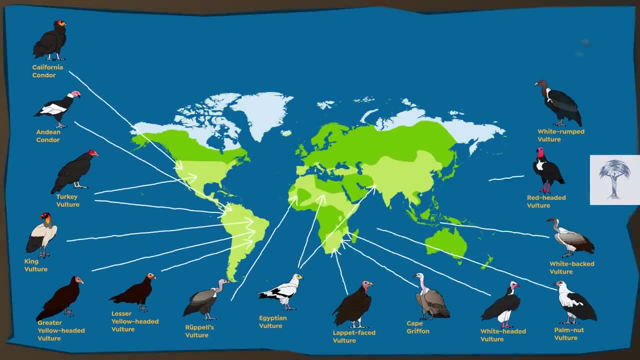 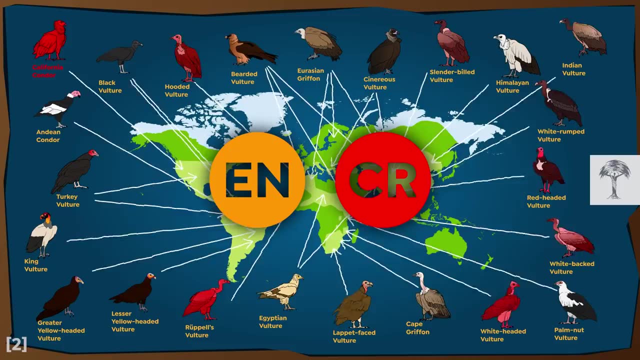 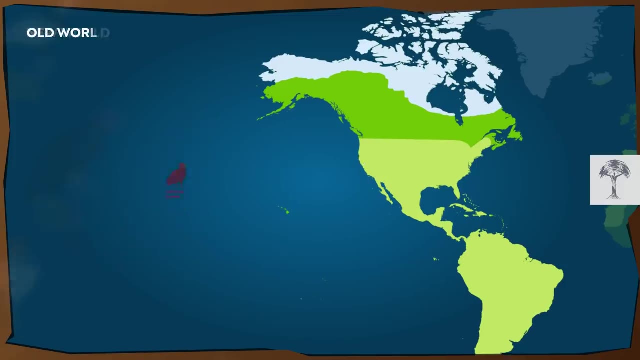 But across the world vulture populations are under threat. Of the 23 species on the planet, three are endangered and further nine are critically endangered. One of these, the California condor, is found in North America. The rest are so-called Old 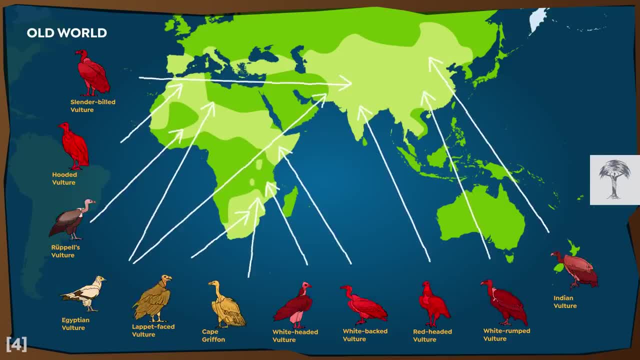 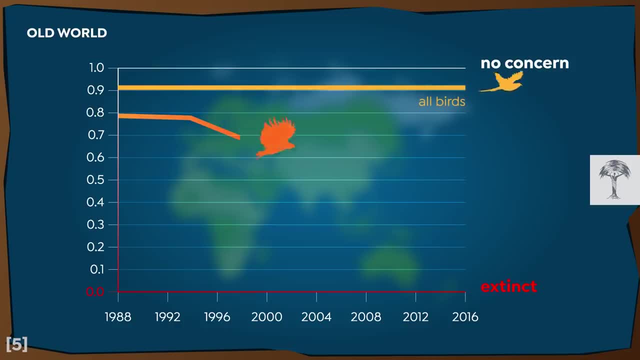 World vultures found across Africa and Eurasia. In fact, compared to all birds worldwide, Old World vultures are declining at an alarming rate. But why? One of the main reasons is… they're being poisoned. In the 1990s in South Asia, an estimated 90% of the vulture population was wiped out by 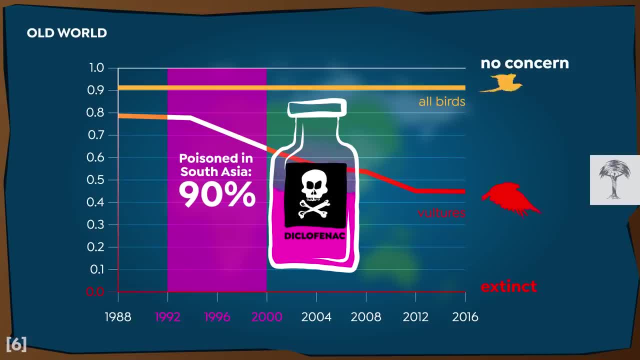 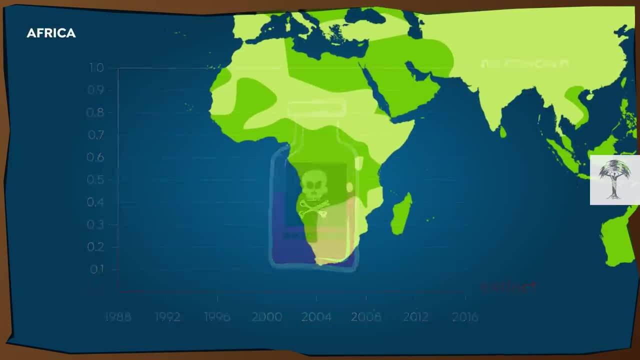 the medication diclofenac. The dead cattle they'd been feeding on had been given the medicine, which is highly toxic to vultures, And across Africa, but especially in the South and East, vultures are also dying in large numbers. 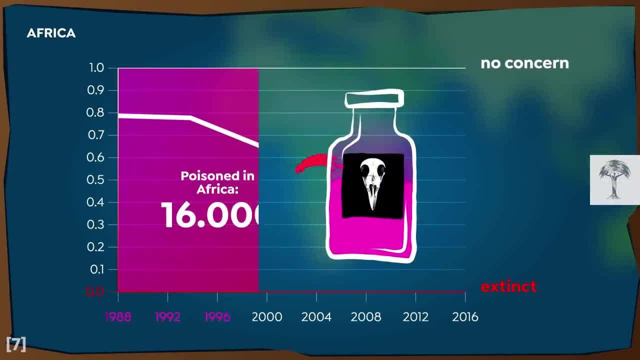 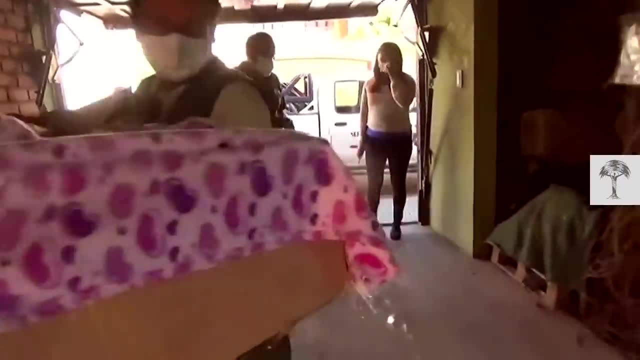 Official data suggests that more than 16% of all vultures die in large numbers in the South and East. More than 15,000 have been poisoned since the 1960s. Sometimes it's accidental. This Andean condor is thought to have been poisoned by drugs. 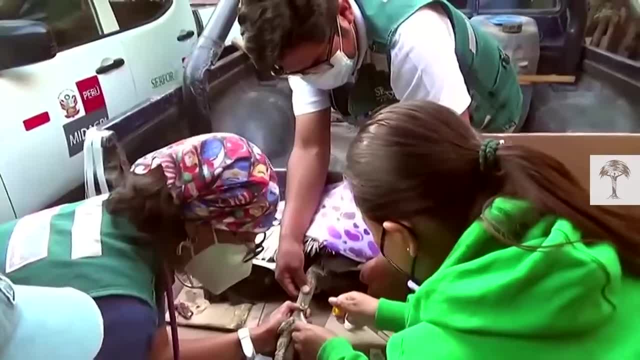 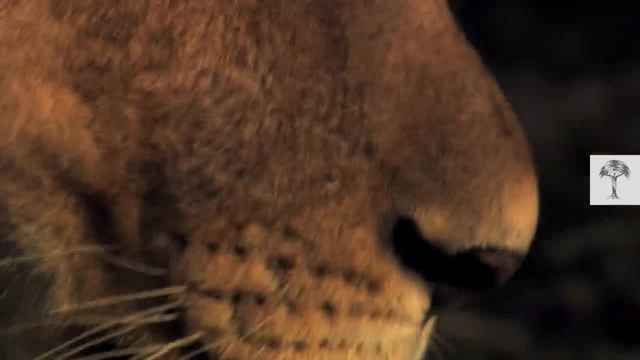 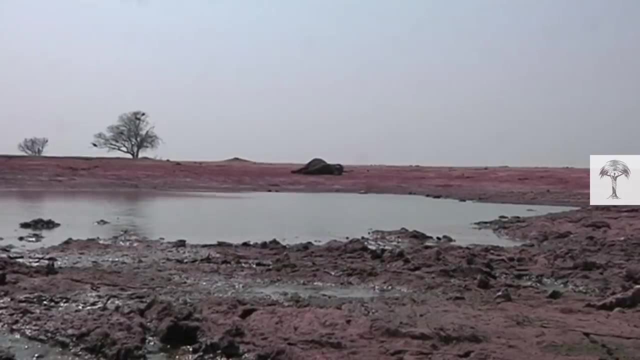 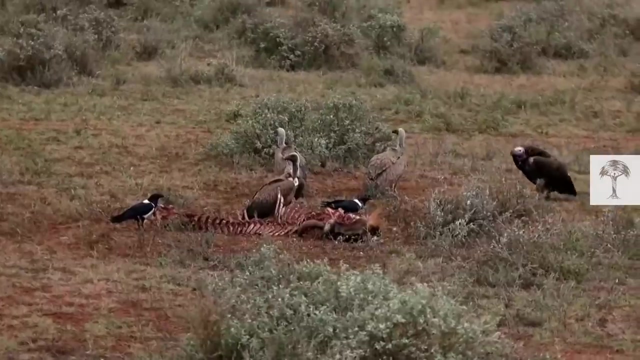 given to cattle. Its condition is fragile. Other farmers or herders often poison dead livestock to keep away dangerous predators such as lions, But other times it's deliberate. In 2013,, 500 vultures died in Namibia after feeding on an elephant carcass poisoned by 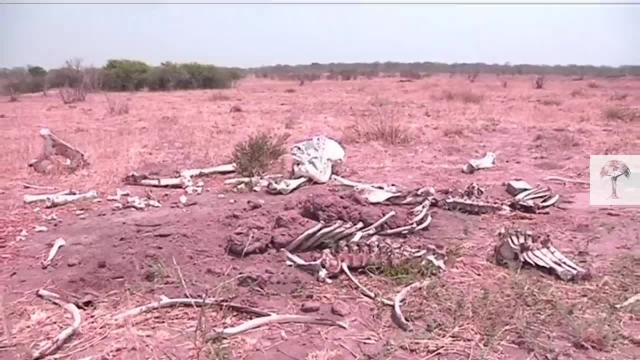 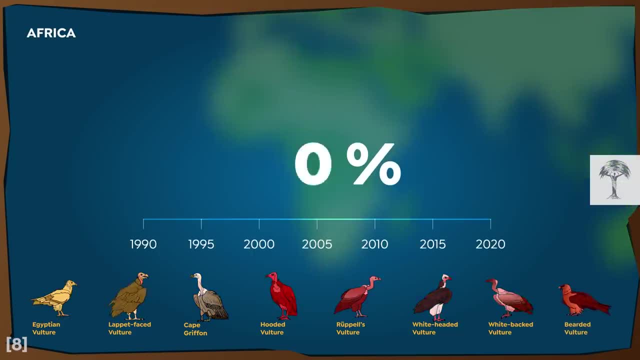 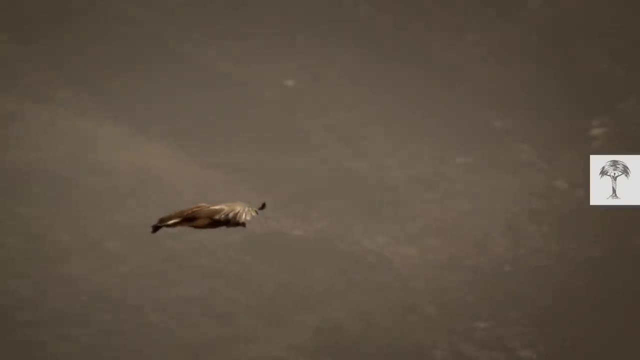 poachers. As a result of all this, the seven most endangered vultures in Africa, plus the bearded vulture, which is near threatened, have declined by around 62% in the last 30 years. The number of dead vultures in Africa has declined by around 62% in the last 30 years. 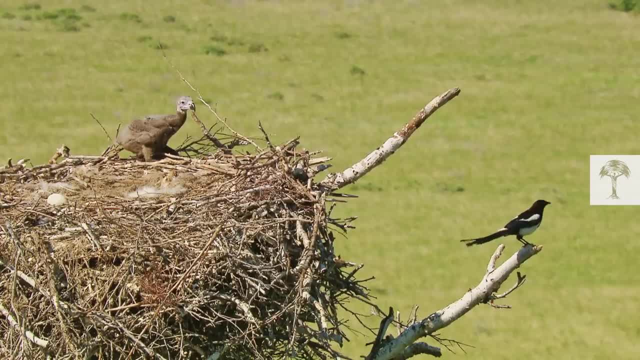 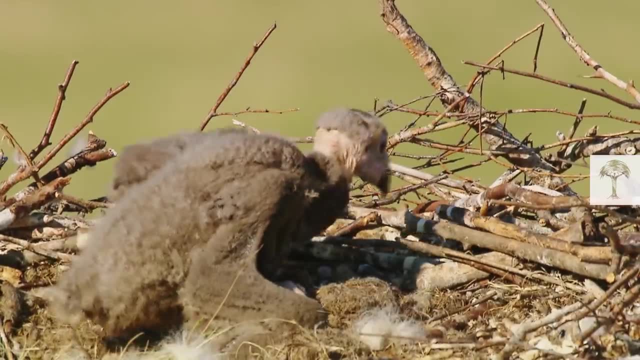 The decimated numbers are exacerbated by the increase in the number of dead vultures in Africa. This is caused by the fact that vultures lay eggs so rarely, just one or two a year. With so few offspring, restoring the population is even more difficult. 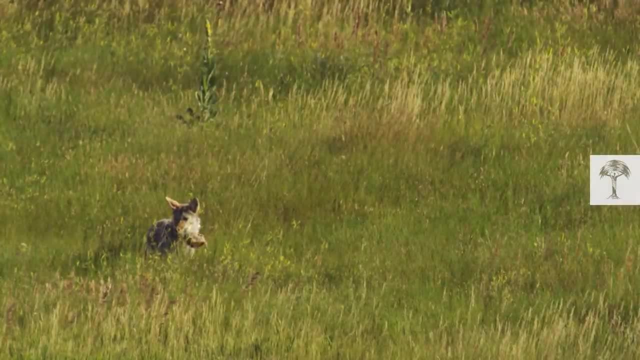 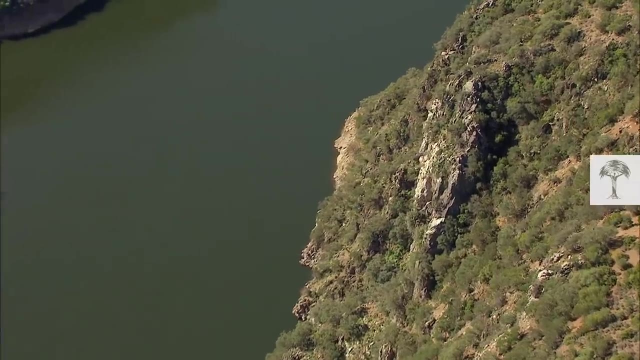 But surely there are enough other scavengers to take over vultures' position in the food web? Well, yes, there are, but that's exactly where one of the problem lies. Another vital role played by vultures is to indirectly control other scavenger populations. 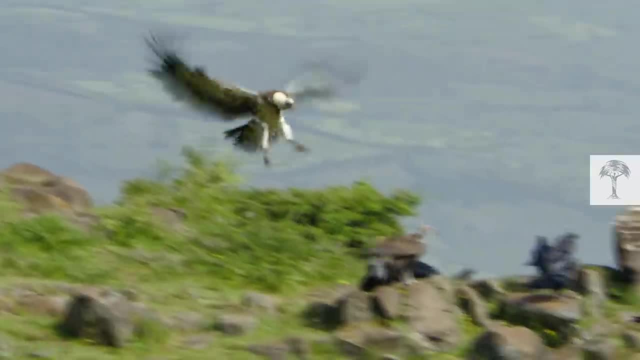 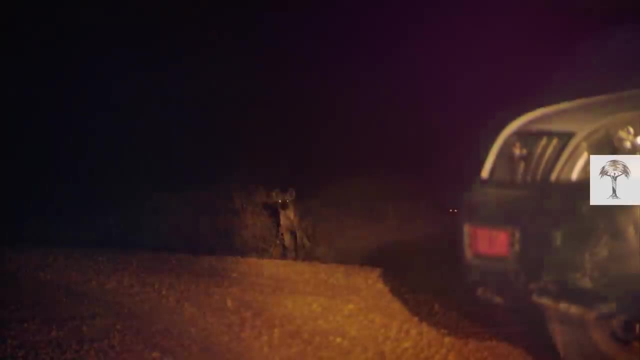 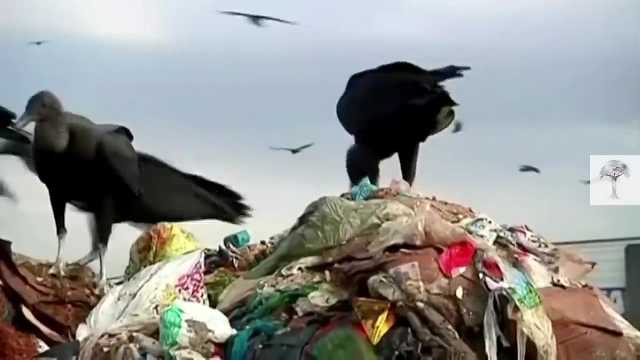 by reducing the amount of food available. And, as we saw earlier, some of these scavengers are also predators, like hyenas or lions, which can threaten humans and livestock. Many of them also spread diseases, as only few species can break down toxins as effectively. 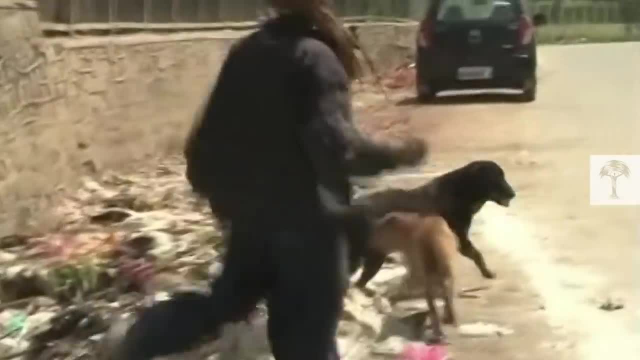 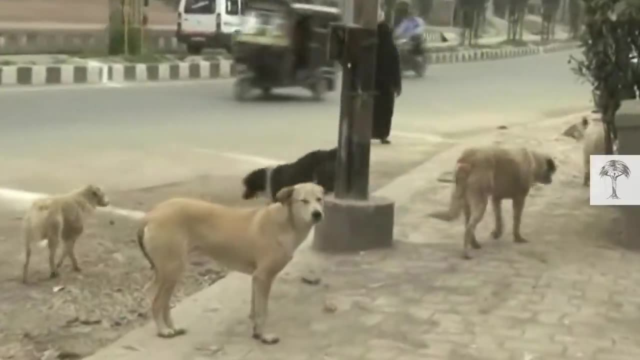 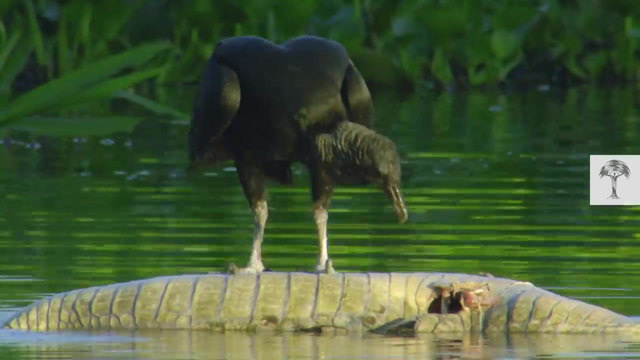 as vultures can. The number of human rabies cases in India rose dramatically when the vulture population declined, thanks to feral dogs that took over scavenging duties and spread the disease. Vultures don't just remove toxic bacteria from the ecosystem, but they are also very clean creatures. Their bald heads prevent rotting flesh from sticking to their feathers and falling off elsewhere. They also urinate on their legs to cool down and clean off bacteria, And by flying long distances they can spread nutrients far and wide. Vultures are also very clean. 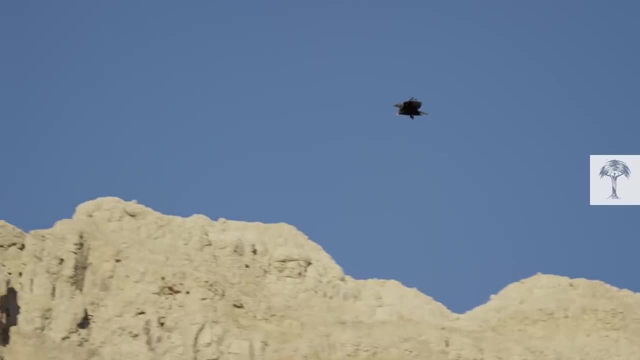 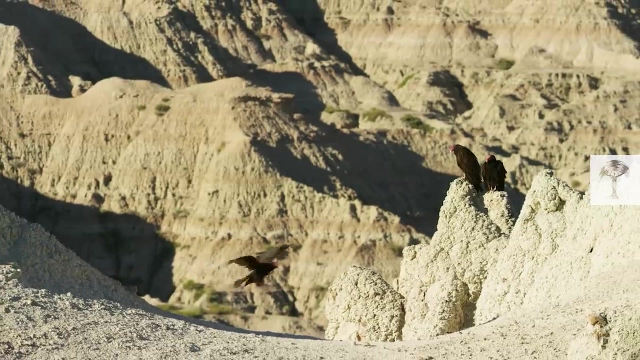 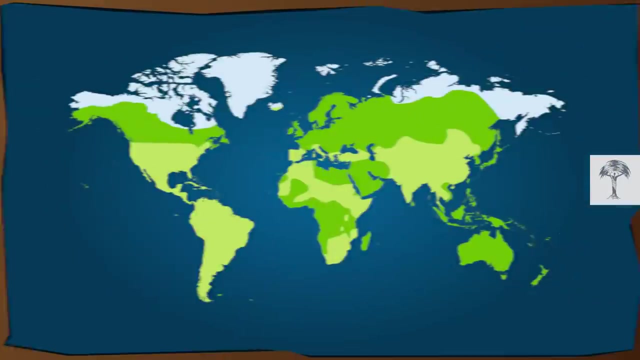 Recently, one young vulture was recorded flying nearly 1,800 kilometers in just three months. In fact, vultures are so crucial to ecosystems that they are known as keystone species. Poisoning isn't the only thing that's killing vultures in Africa and Eurasia. 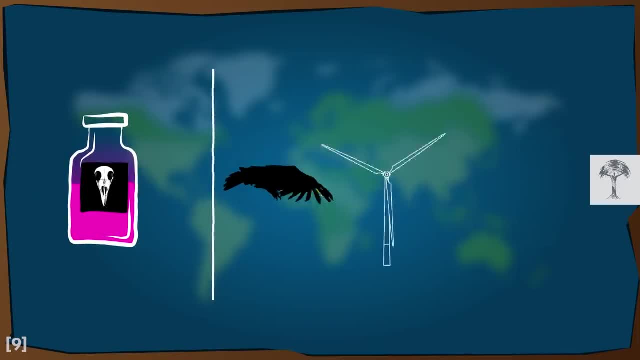 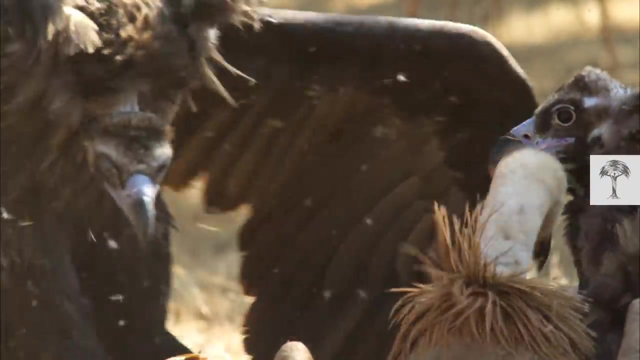 Windmills and power lines cause fatal accidents because vultures tend to look sideways rather than straight ahead And…. The trade in vulture meat – especially heads and feet, which are used in traditional medicine – also contributes to the decline. The problem is, people don't really understand the true value of vultures.